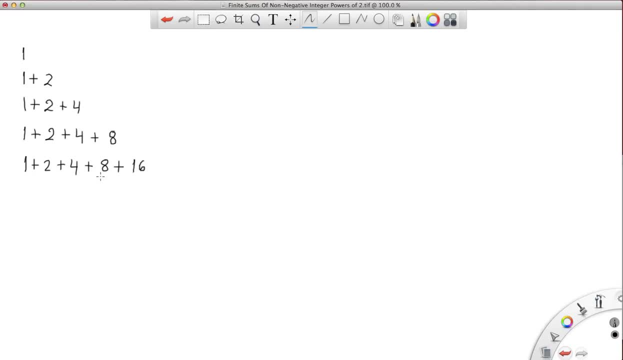 next, power of 2. the only thing we need to do is to multiply the previous one times 2. so here, 1 times 2 is 2, and then 2 times 2 is 4, and 4 times 2 is 8, and so 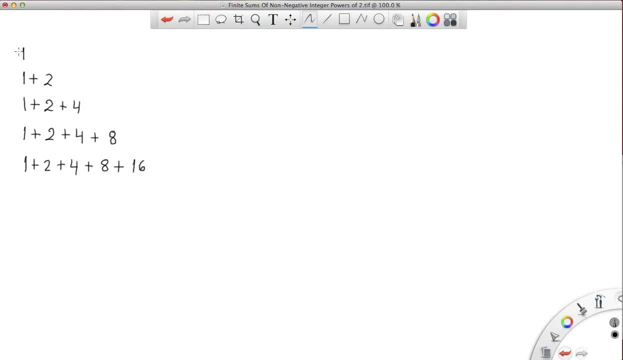 on. and the first number where 1 is 2 to the 0. now let's record the results. if we only have the number 1, that's it 1. when we add 1 plus 2, we get 3. when we add 1 plus 2 plus 4, we get 7. then here we have that. 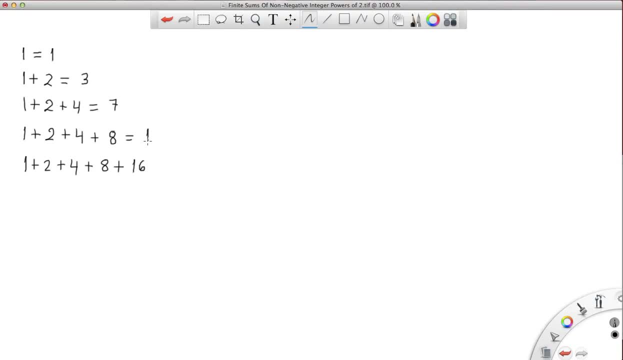 same sum plus 8. so 7 plus 8 equals 15. and then in these sum 1 plus 2 is 3 plus 47 plus 8 is 15, and 15 is 16, and 16 is 15 plus 16 equals 31. now notice this relationship here between the result of: 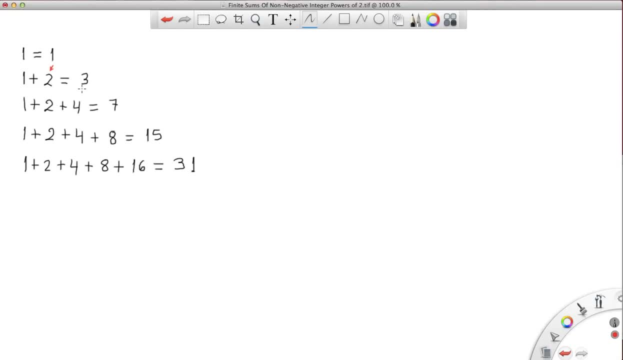 the sum in a given row with the last power of 2 that we are adding in the next row, see 1 and 2,, 3 and 4,, 7 and 8,, 15 and 16. there is a difference of 1. the result of the sum is always one unit less than the next power of 2. 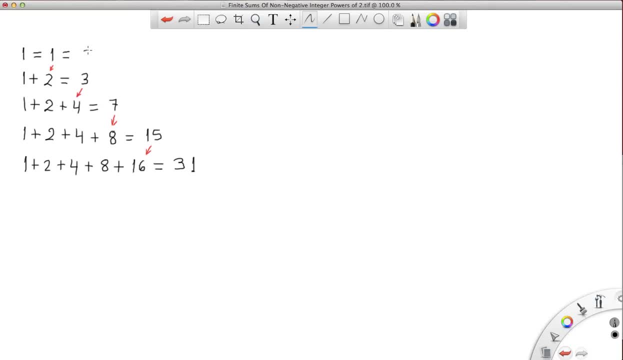 one is 2 minus 1, then three is 4 minus 1,, 7 is 8 minus 1,, 15 is 16 minus 1, 31 equals 32 minus 1, and so on. this just keeps going when we start adding powers of 2 like that. 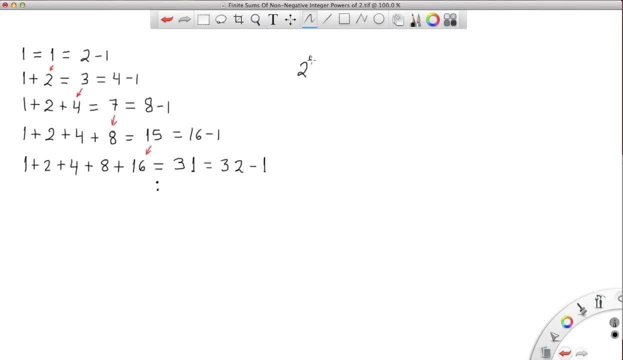 from 2 to the 0,, which is the number 1, and then increasing 2 to the 0,, plus 2 to the 1, and so on. we are always going to get one unit less than the next power of 2. 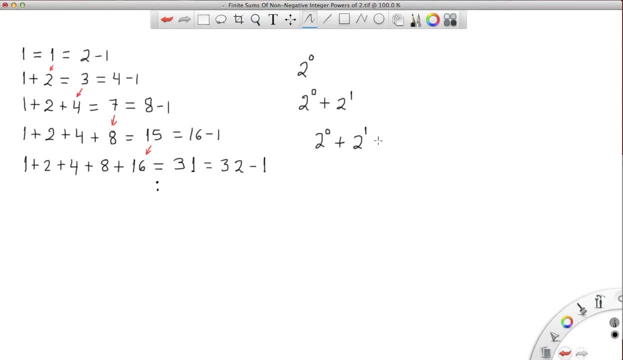 and that will be the next power of 2 relative to the last one we included in the sum. so 2 to the 0, plus 2 to the 1, here we are just rewriting the same thing, but we are making it explicit with the exponents. 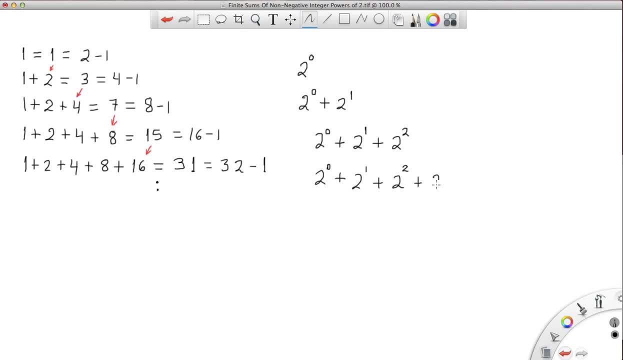 2 to the 2, and then the next one is 2 to the 3. so here we have just the number 1, which is 2 minus 1, but 2 is 2 to the 1,, so we can rewrite this as: 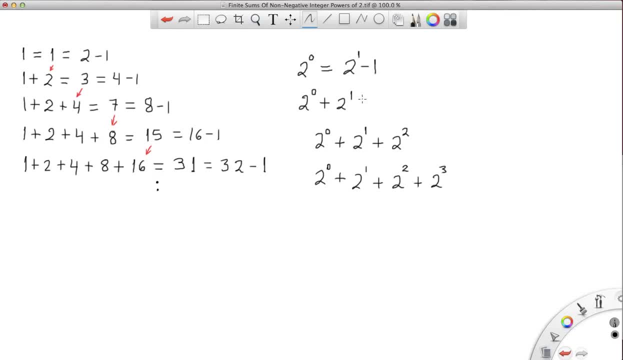 2 to the 1, minus 1. here we have 1 plus 2, which is 3,. 3 is 4 minus 1, so this is 2 to the 2 minus 1. here we have 1 plus 2, plus 4. 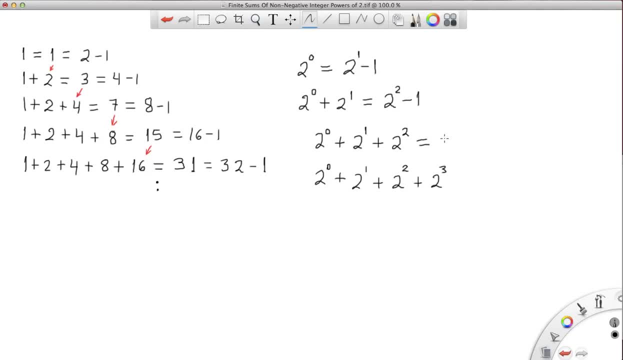 so that one is 7, and 7 is 8, minus 1, but 8 is 2 to the 3. see the next power of 1, the next power of 2, minus 1 here. the next power is 2 to the 4. 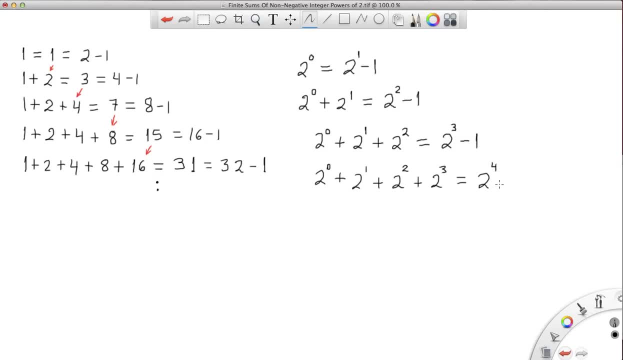 which is 16, and then minus 1 is 15, which is the result of that sum. so let me write the notation in extended form. for any arbitrary number, we are going to use a letter to represent the exponent where we are going to finish. 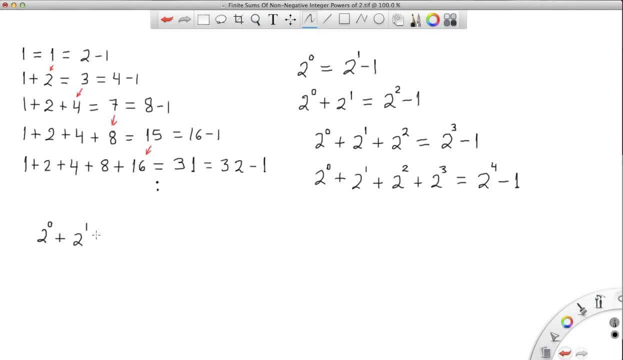 so 2 to the 0, plus, 2 to the 1 plus, 2 to the 2 plus, and then we just write dots to indicate that the sum continues and this sum is going to stop at a power of 2 to the exponent n. 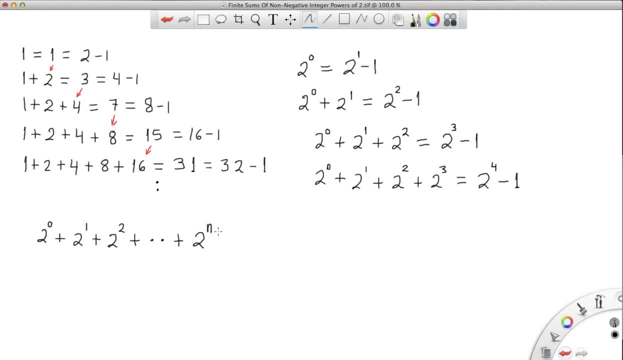 where n is an arbitrary number. so that's the last power of 2 that we are adding. and then here we have the sum. the result of the sum is going to be one unit less than the next power of 2, so we increase the exponent by 1.